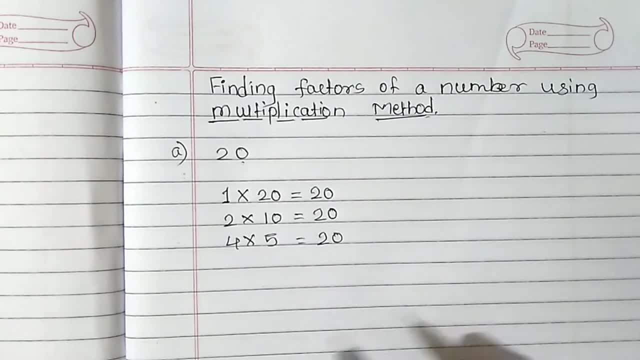 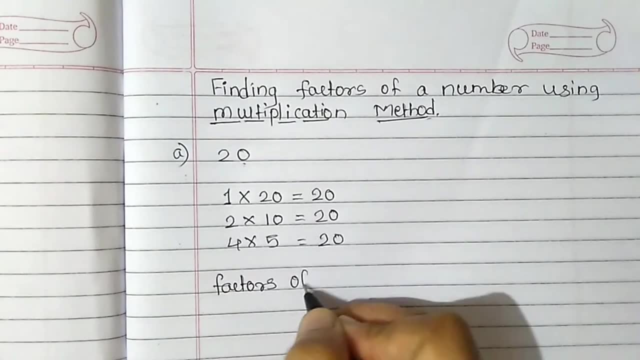 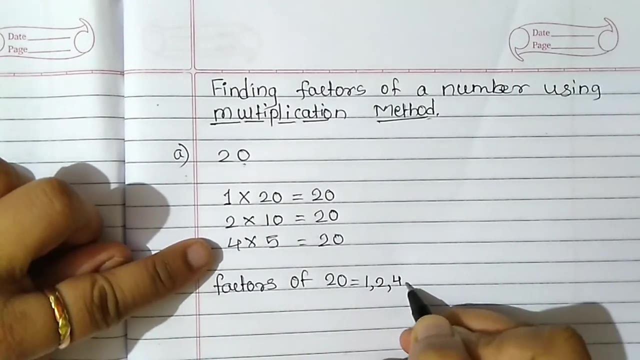 Correct, So now we will stop at this. Ok, So these are the factors of 20.. How do you want to write: Look at this. Factors of 20 equals to Look at this: 1, 2, 4, 5, 6. 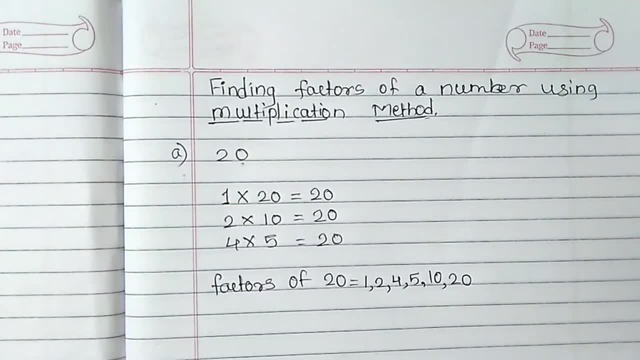 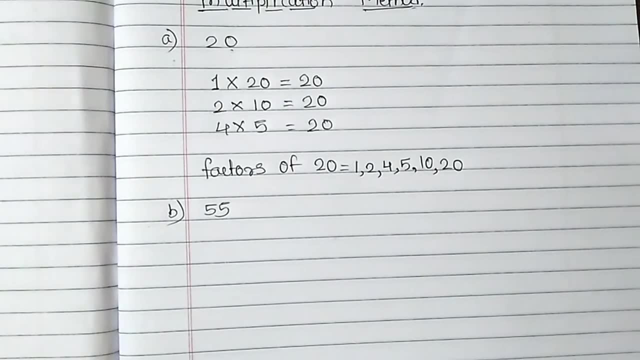 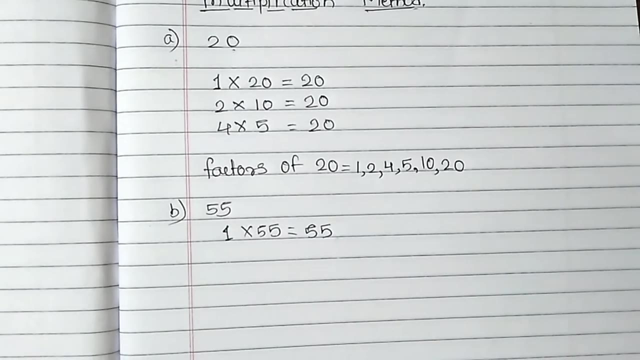 10 and last 20. ok, next be example 55. again same 1 into 55, 55 next to keep us doing it can up to pataki last May: 0, 2, 4, 6, 8, me hey, 50, power is not divisible. 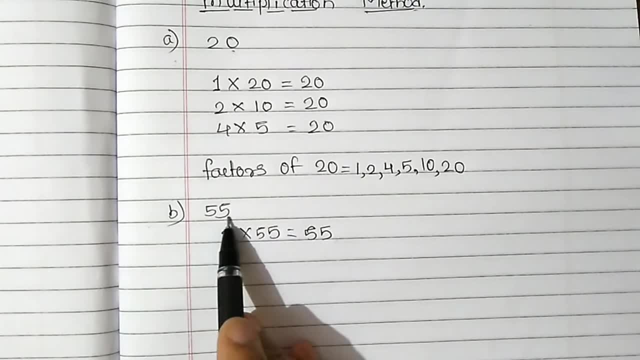 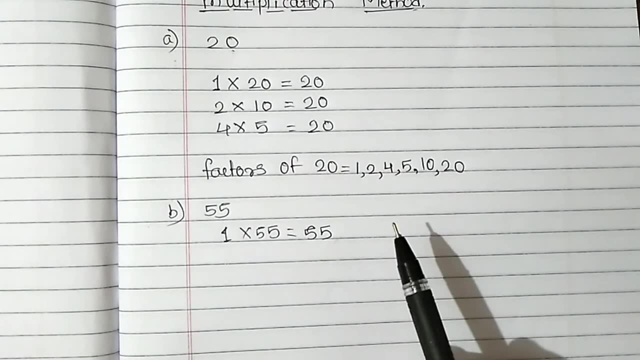 by 2, next 3 k, pas jayenge, 5 plus 5. you tell what I hate. the 3k table may be named at the head to 4 k, pas jayenge the king. 4 k table, maybe 55 any other. 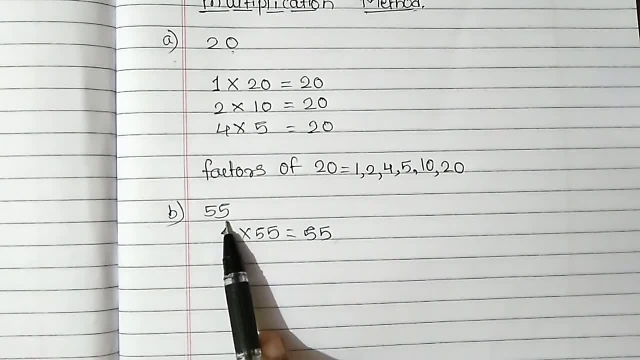 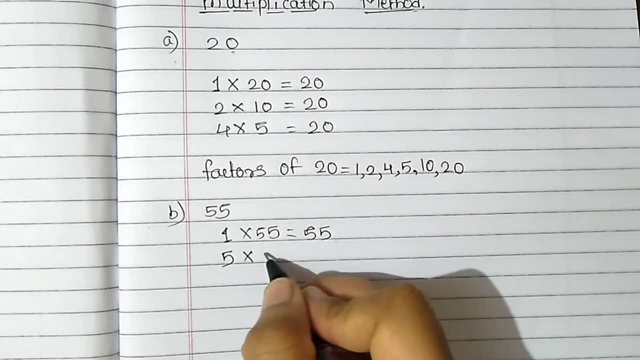 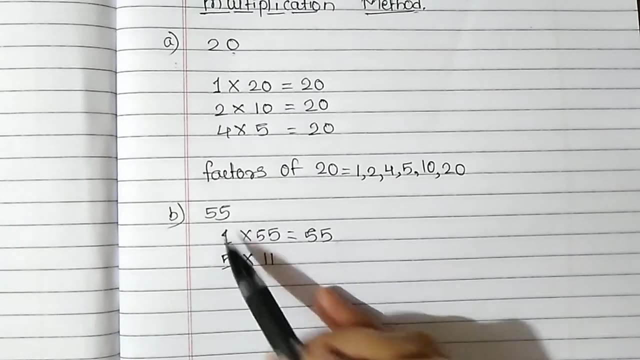 theorem jayenge, 5 k, pas to last May. 5 a matlab, yes, yep, I could table may at the head. so for you cook on, say number, say multiply, connect about at the head: 11, 11 files of 55, a girl of kune. he put the: hey see, top care, okay, 50 pi co pi. 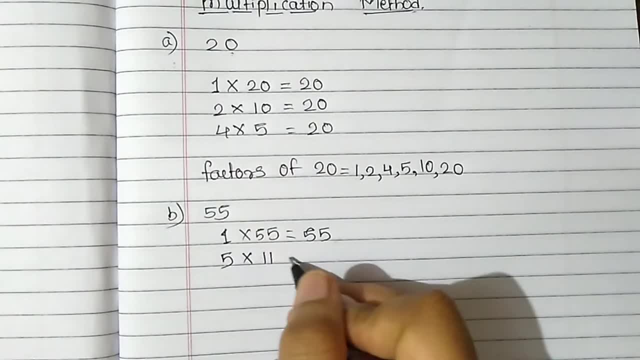 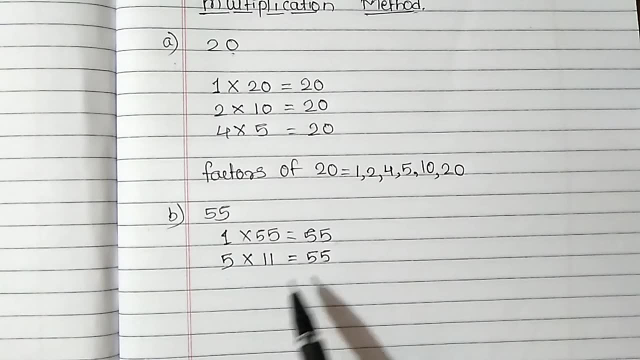 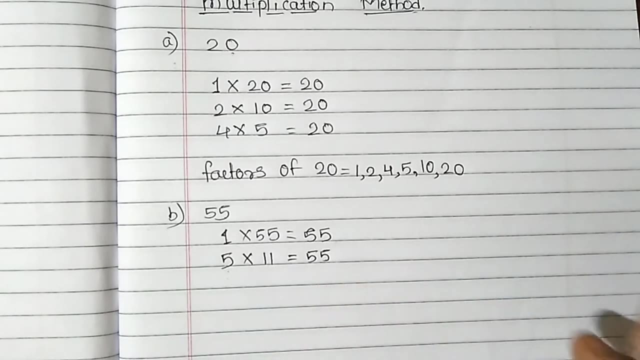 say: divide Karthik o kita approval a level. answer me later to your paper. take up next six KB. table many other seven k-98, k-98, k ne, 11 kata Hillary, 11 files of 55. the factor whamma a pie already mill chuka. Hey to him. yay, peace course top. 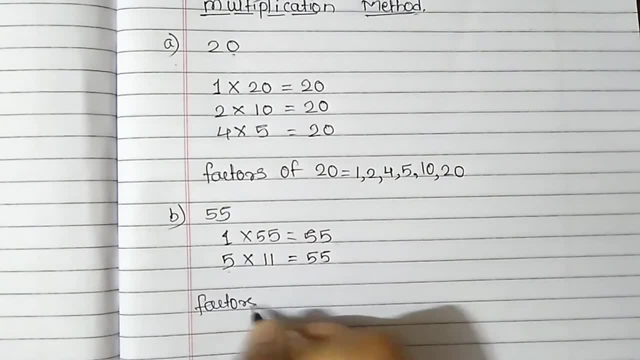 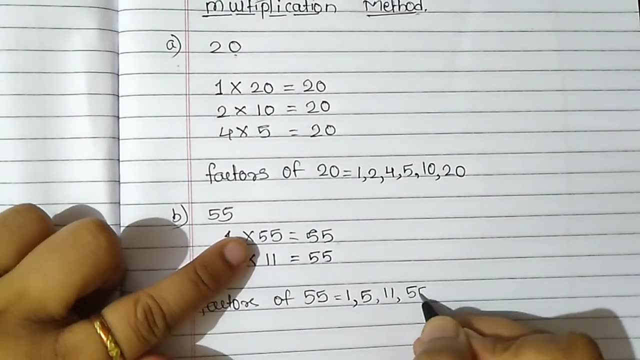 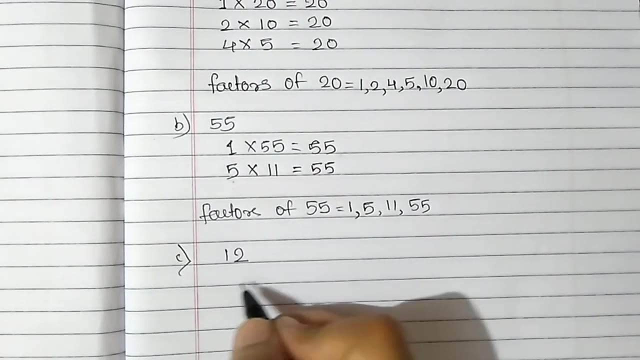 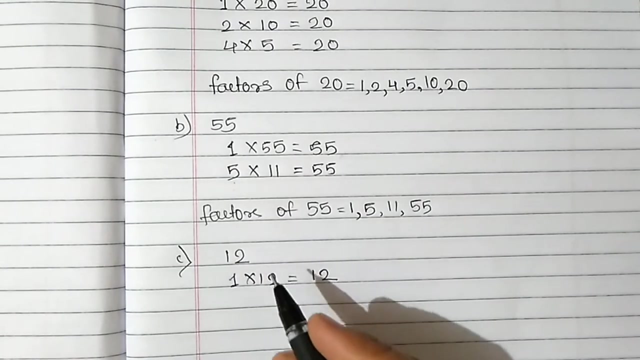 current. okay, so yeah, I pay up cup. I never answer a eager. factors of 50 pi equal to 1, pi 11 and 55. ok, Next C, 12. Same 1 into 12 Equals to 12. Last is 2 means it comes in 2's table. 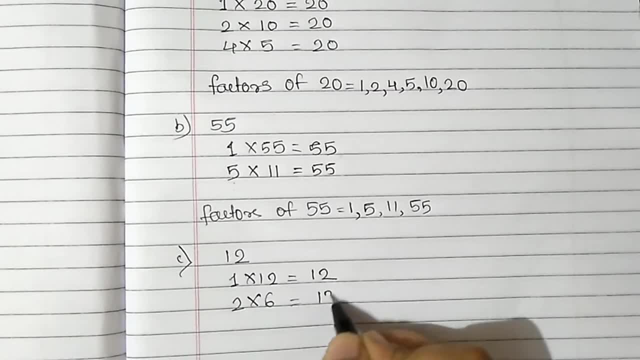 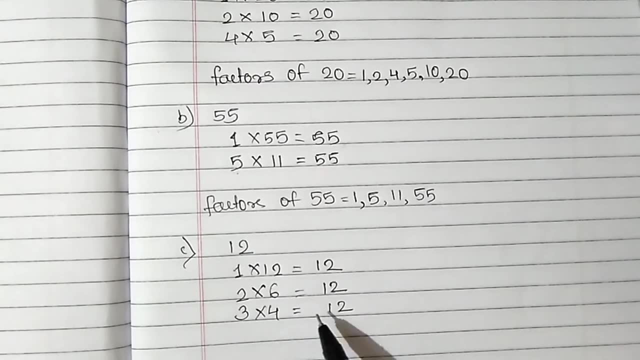 2 into 6. 2, 6's are 12, Next 3, 4's are 12, Next 4: 3's are 12. Then it doesn't come in 5's table. 6, 2's are 12. The vector we have already got. 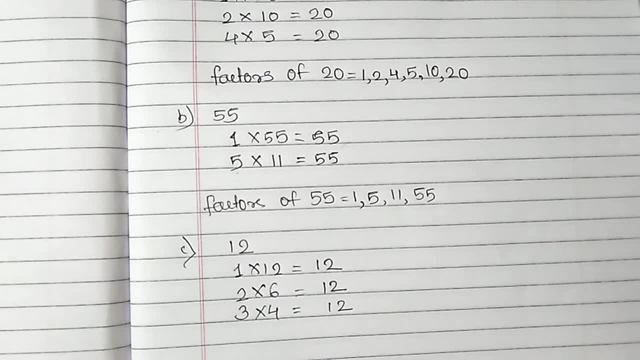 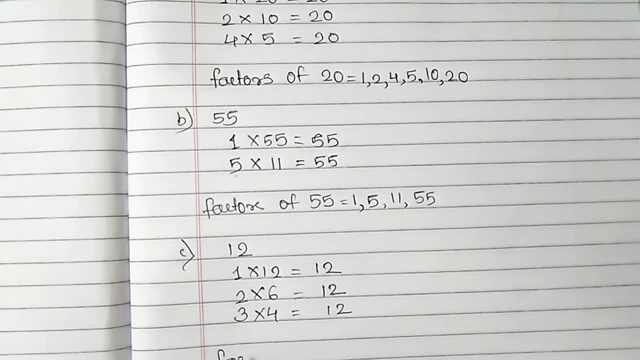 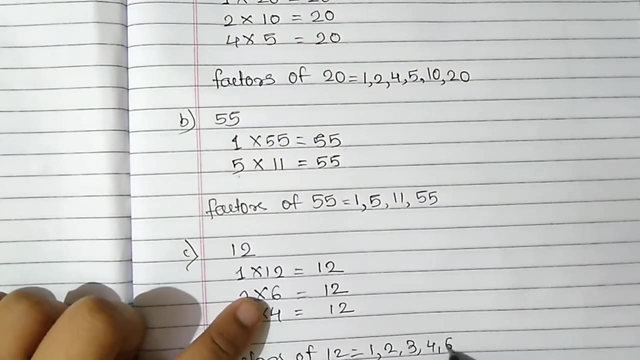 So we don't have to write 4. 3's are 12. Again, like this, We will stop here. So here, Factors of 12 equals. to See, I am writing sequentially 3, 4, 6 and 12. Ok, Let's solve one more example. 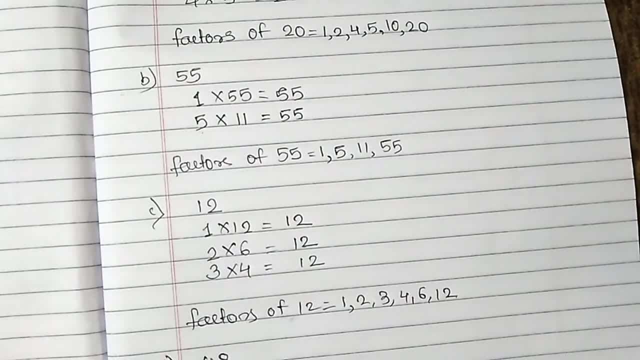 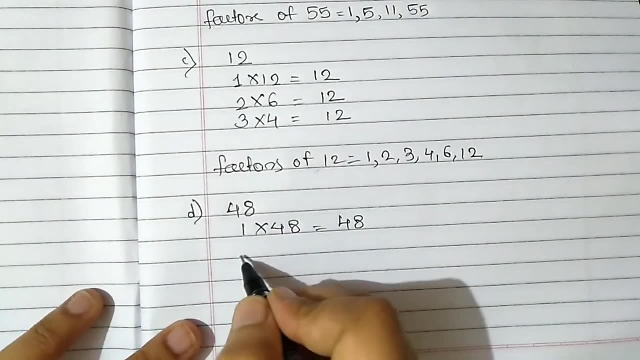 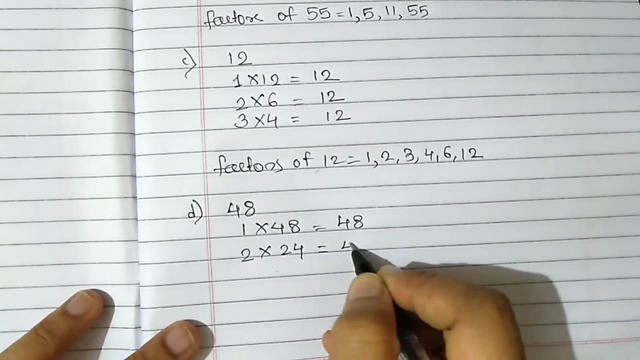 Then we will stop. Let's take 48: Same 1 into 48 Equals to 48. Next Last is 8. means it comes in 2's table. 2 into what number? After multiplying, it will come 24. Ok, 12 comes in 3's table. 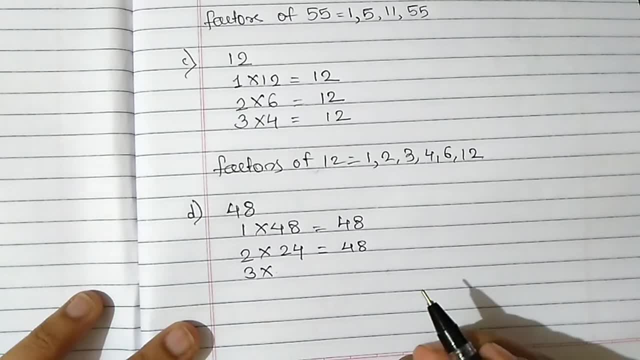 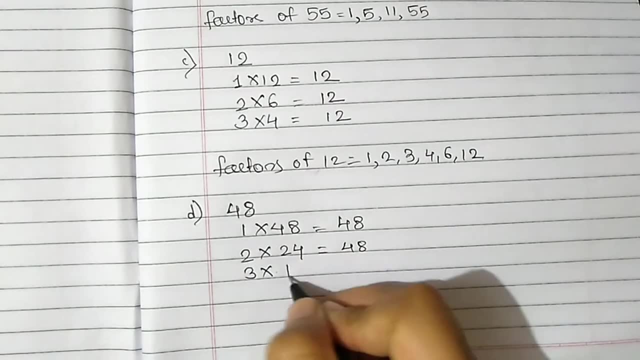 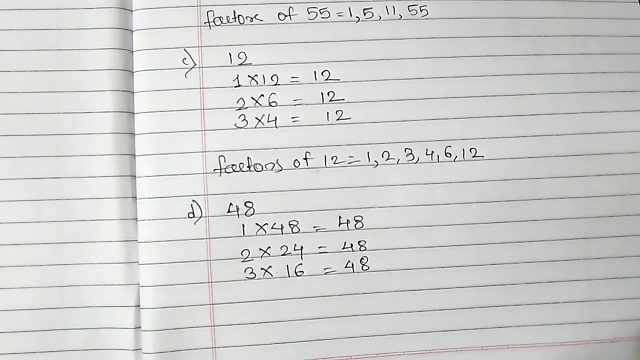 Means this 48 also comes in 3's table. Ok, So after multiplying 3, into what number 48 will come? Yes, 16. I have already told you. If you don't get it directly like this, Then what will you do? You will divide it, Ok. 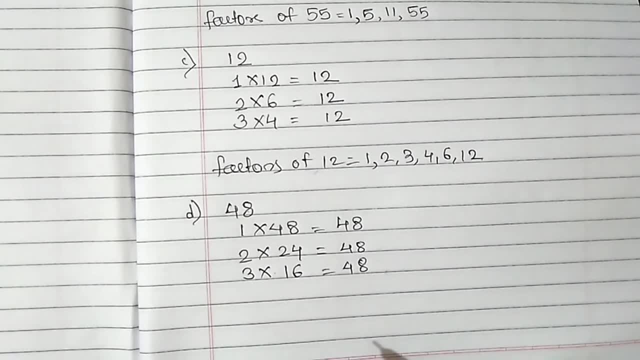 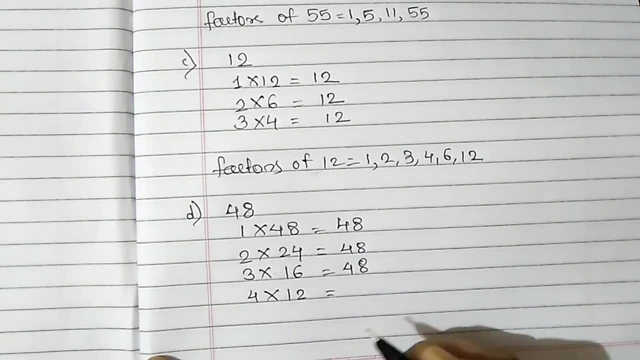 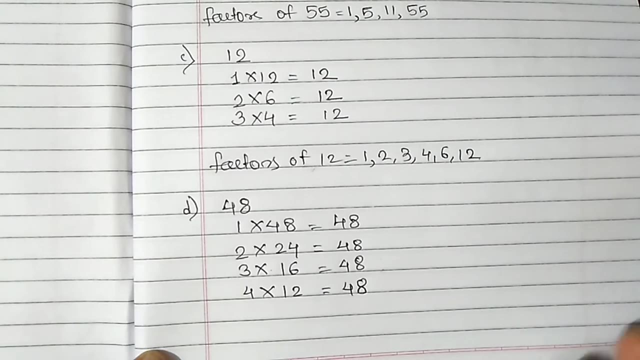 Next We will go to 4 now. So 48 comes in 4's table, Comes 4 into 12, 12 for the 48. Next Doesn't come in 5's table: 6, yes, 6 into 8. 6 8's are 48. 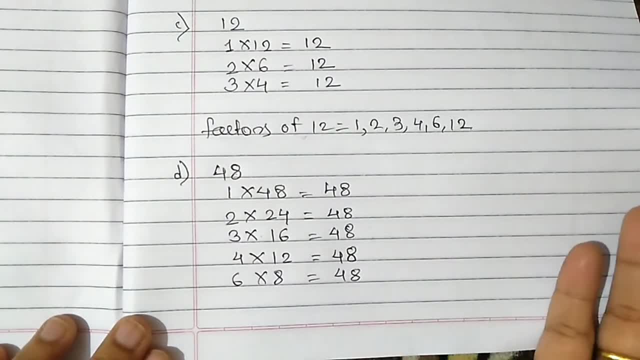 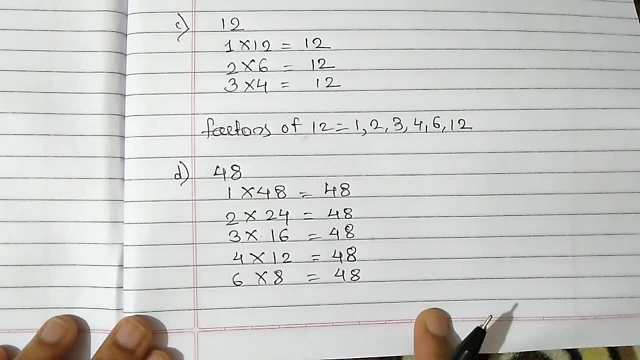 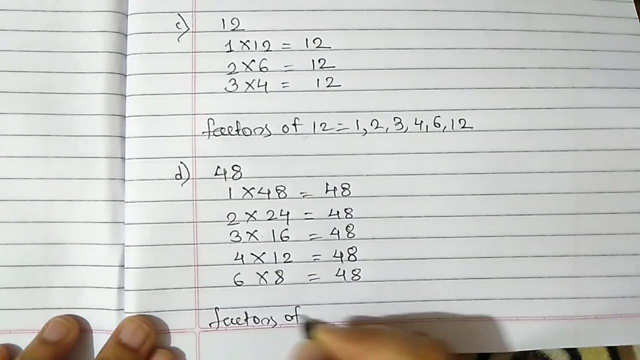 Next Doesn't come in 7's table 8 comes in 8's table 8, 6 and 48. So you have already got 6 factors, So do we need to go ahead? No, So we will stop here. So right here, Factors of 48 equals to: 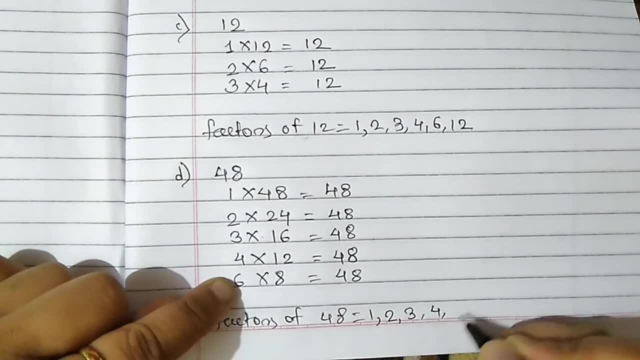 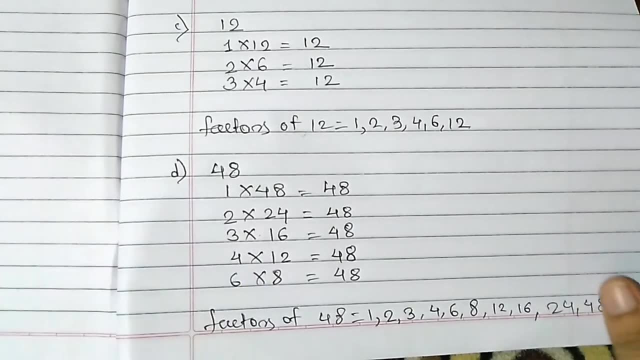 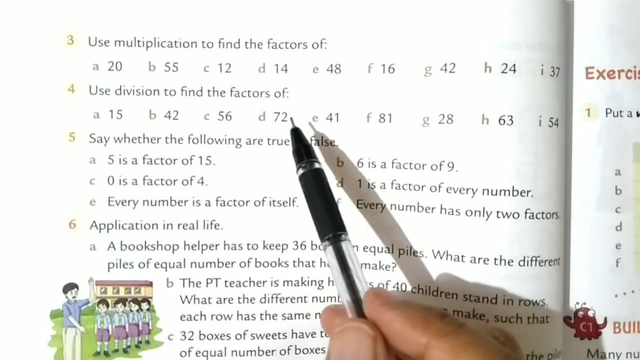 1, 2, 3, 4, 6, 8, 12, 16, 24 And 48. There are many factors of 48 Means. look at 48. there are many tables. It comes in many tables. Ok, So, students, How do you find factors of multiplication method? 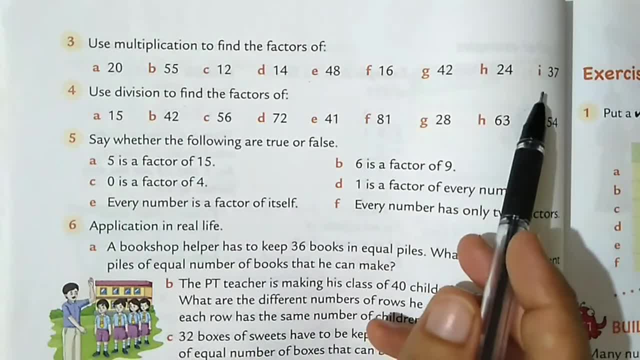 Have you understood well, Very good, So now you have to solve this whole equation. Thank you.